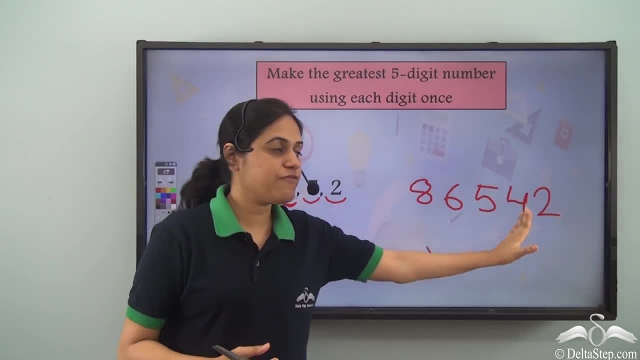 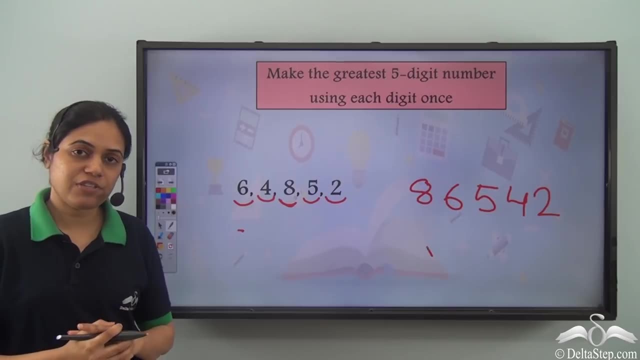 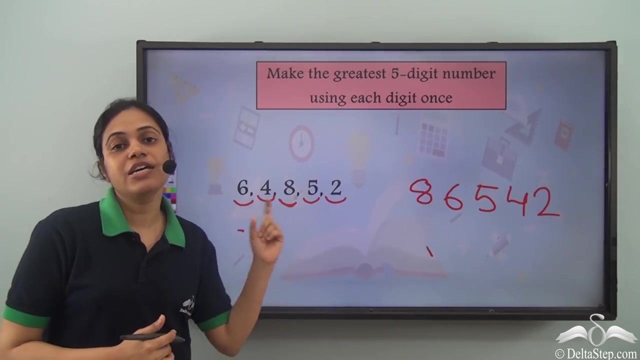 is the greatest five-digit number: 86542.. This is the greatest five-digit number that I can make using these five digits. There cannot be any number greater than this which we can make using these five-digits just once. So why is this happening? Why are we arranging the digits in descending order? 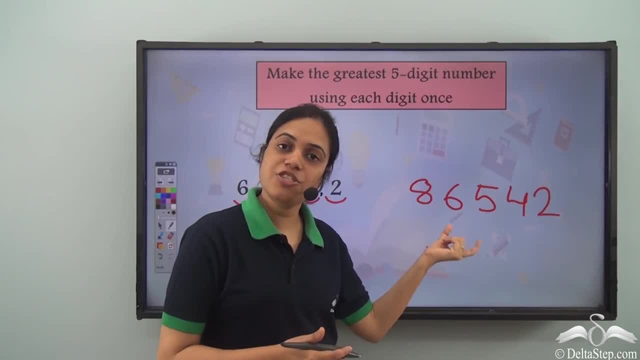 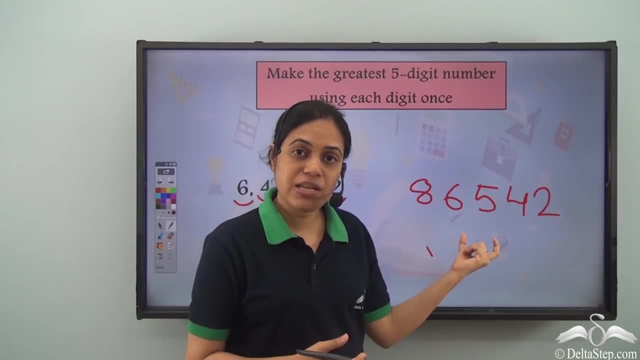 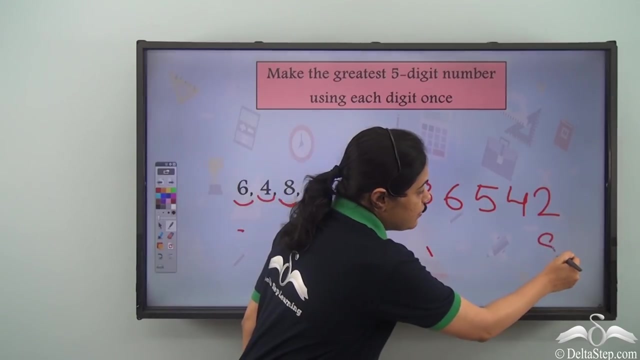 Because I know that if a digit is placed to the left, its place value is more. So I want to make the largest number, So I want the highest digit to have the highest number, So I have more place value. If I write 8 here, then it will be 8 once. But if I write 8 here, 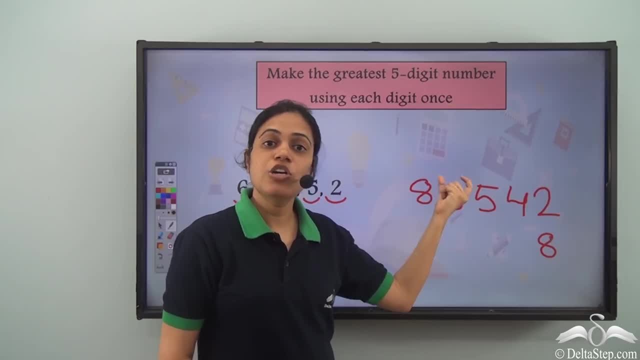 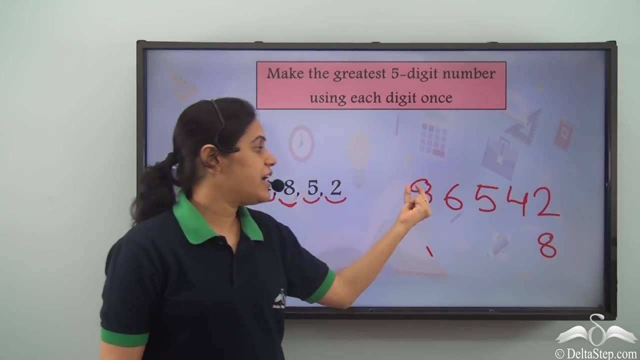 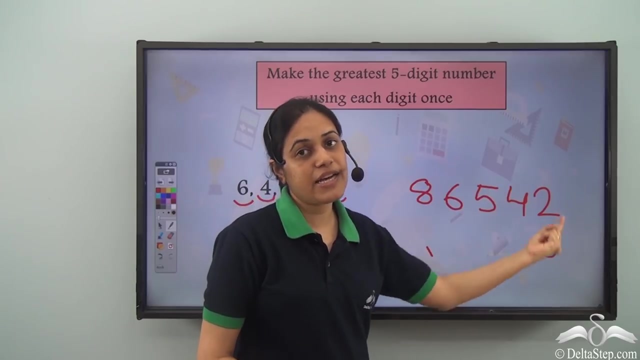 it will be 8 in the ten-thousandths place. So it stands for 80,000.. And this 8 just stands for 8.. So I write the highest or greatest digit first, then the next, then the next, then the next, and so on. 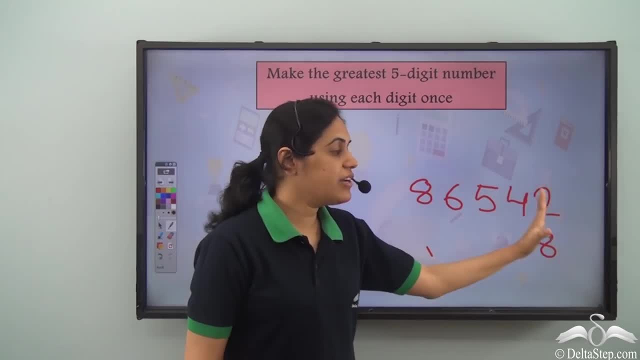 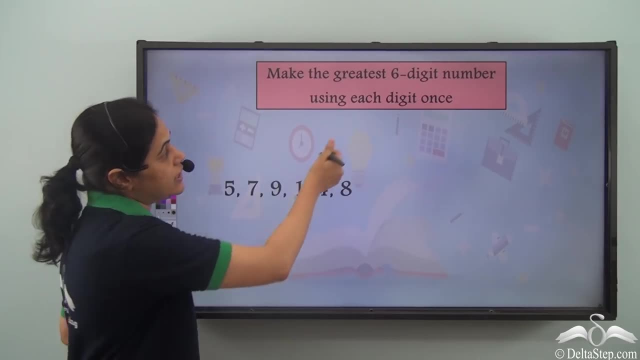 So if I want to make the highest or the largest number, I arrange the digits in descending order. Now we need to make the greatest six-digit number using each digit just once. How can we do that? So, once again, because we need to make the 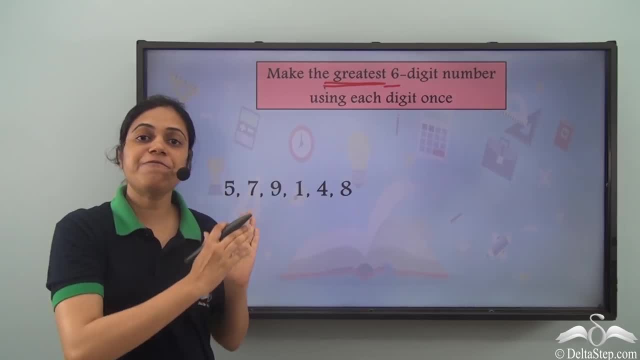 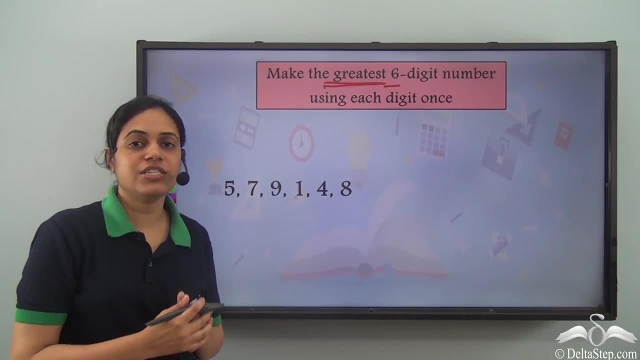 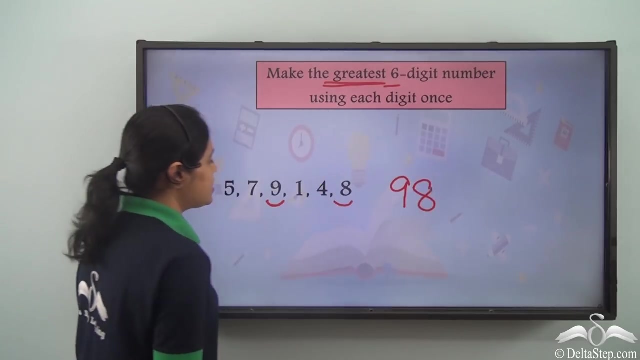 greatest six-digit number. I know that my first digit has to be greatest, So I need to arrange these digits in descending order. This 9 is the largest digit. There cannot be any digit greater than 9.. So I write 9 first, Then I have 8.. So I write 8.. Then I have 7.. So I write 7., Then I have. 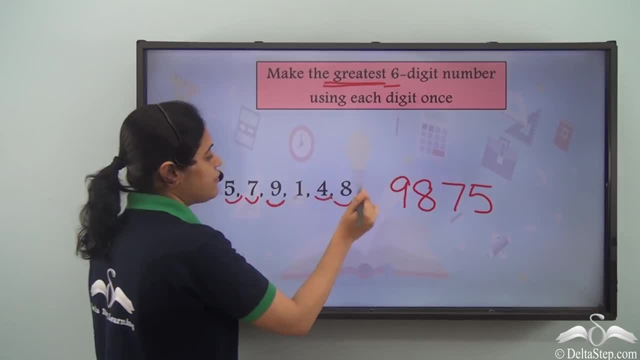 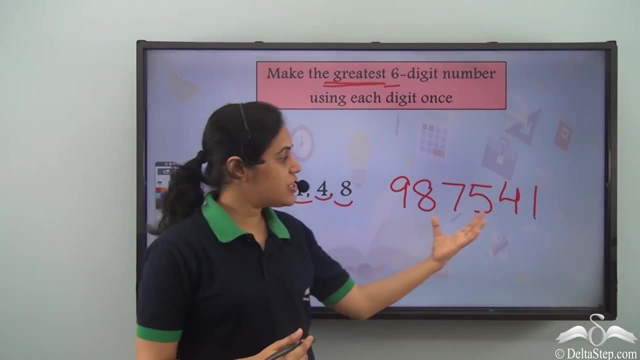 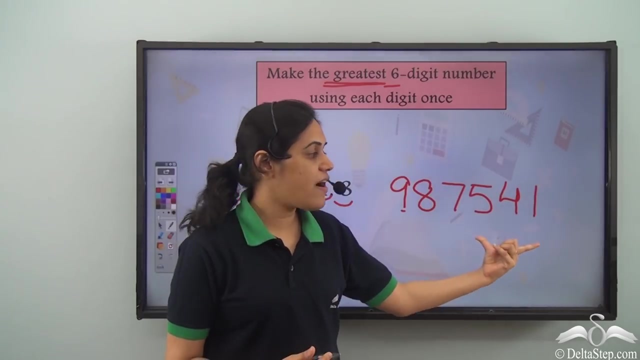 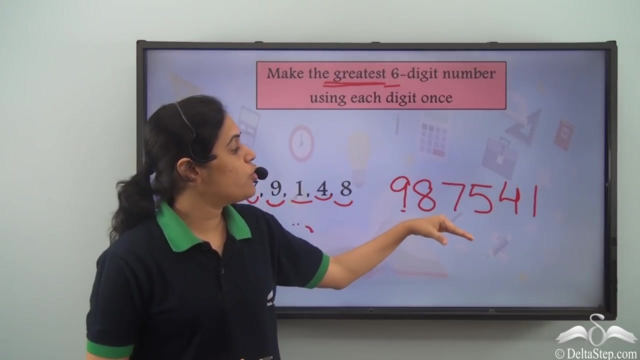 5.. So I write 5., Then 4. And then 1.. So these are the digits arranged in descending order. Now I am not putting commas here. Why? Because this is one number. These are not individual digits anymore. This is a single 6 digit number. So I don't put commas after individual digits. 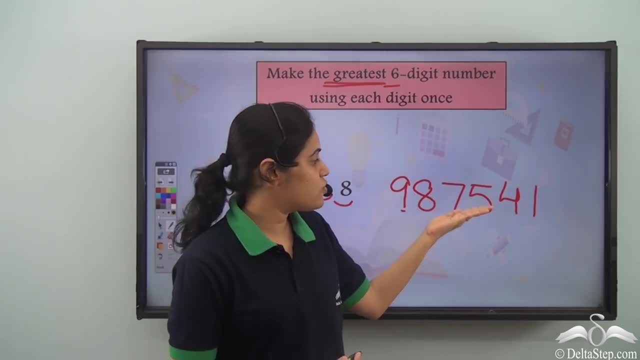 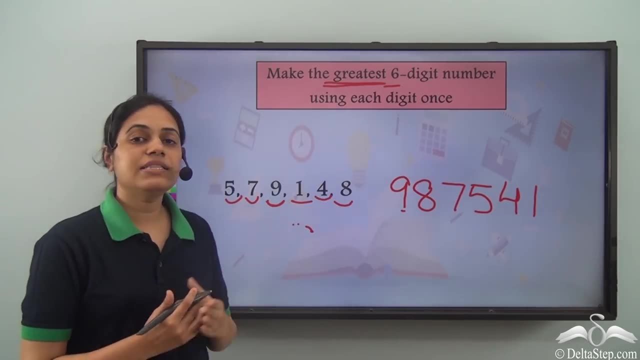 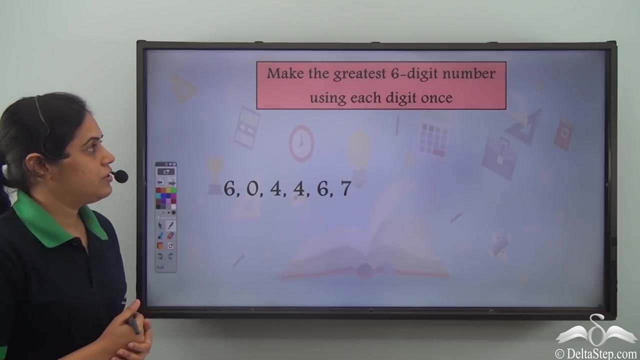 This number is 9,88,000.. 87541.. And this is the greatest 6 digit number that I can make using these 6 digits. So we need to arrange the digits in descending order. So now can you try this on your own, Can you? 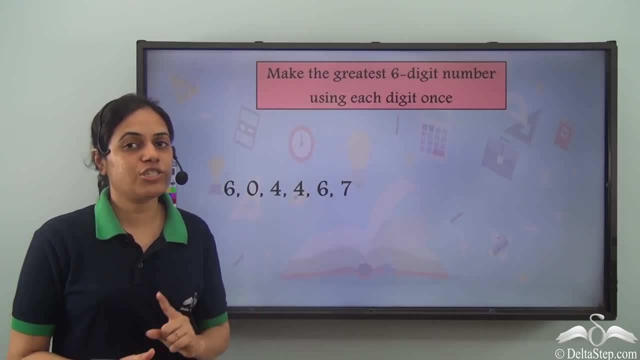 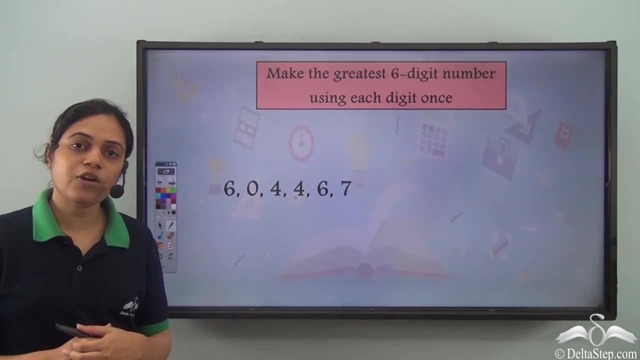 make the greatest 6 digit number using each digit just once. Well, once again, we need to arrange the digits in descending order. We also need to arrange the digits in descending order. We also have a 0 here Now. 0 is the smallest among all the digits, So the greatest digit. 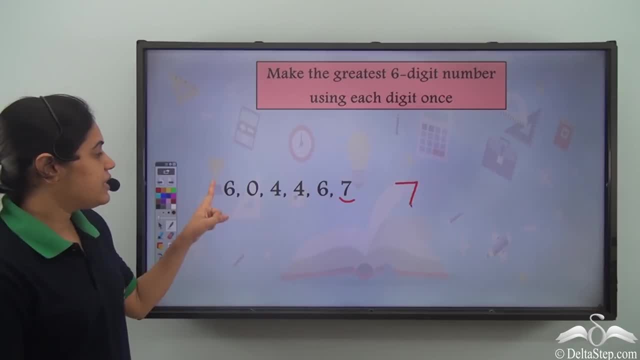 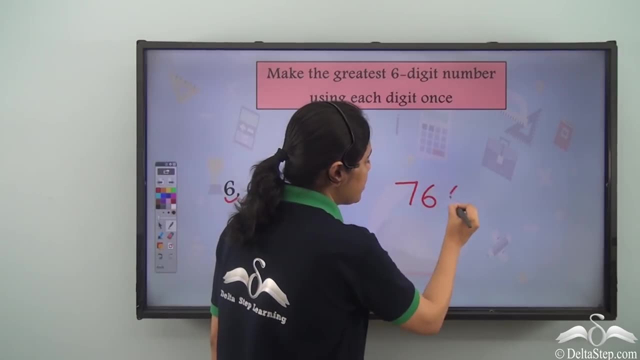 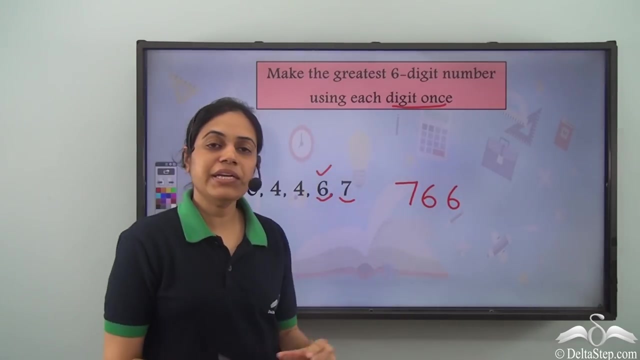 is 7.. I write 7.. Then we have 6 twice, So I need to write 6 2 times. We are using each digit once, But we have been given 6 twice, So I need to write 6 twice. Then we have 2. 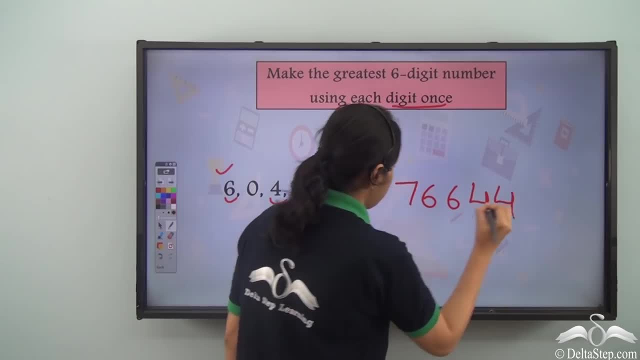 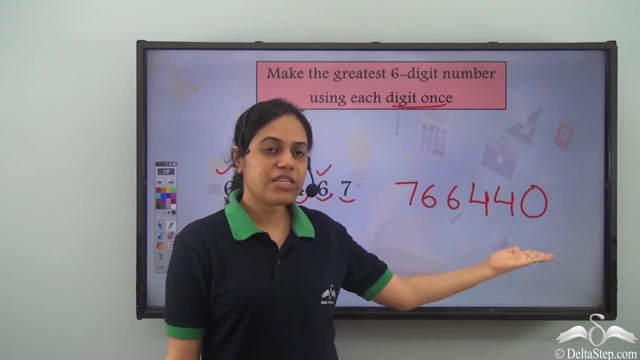 4s, So I write 2.. And then we have 2- 4s, So I need to arrange the digits in descending order. So I write 2, 4s And then a 0. So I have used all the digits. Arrange them in. 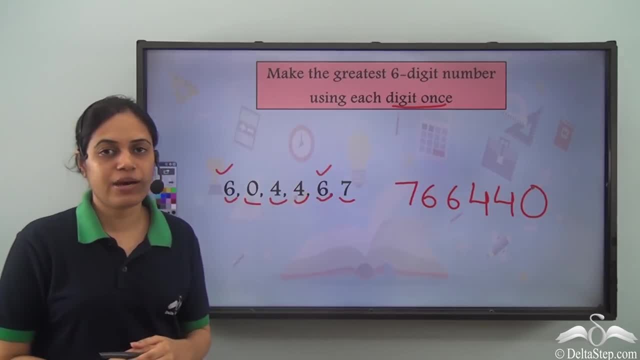 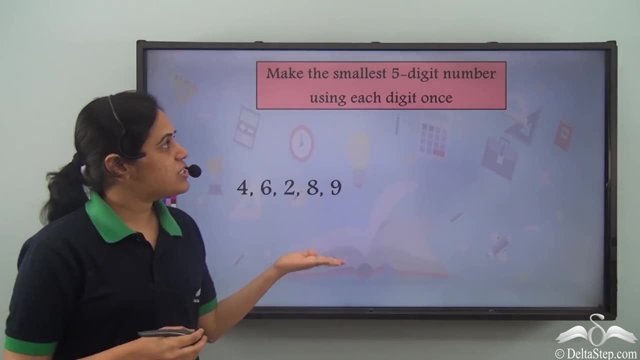 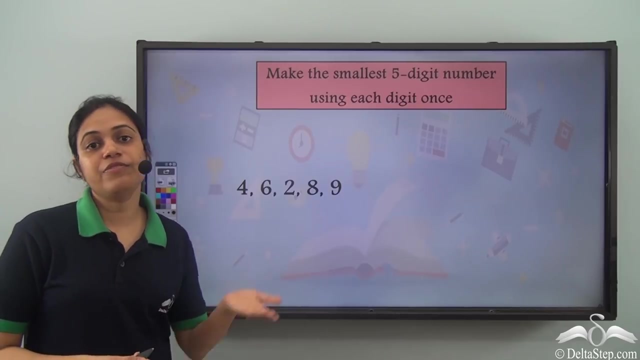 descending order, And this is the greatest 6 digit number that we can make using these digits. Now, what is the smallest 5 digit number which we can make using these digits To make the greatest number? we were arranging the digits in descending order, So we need to 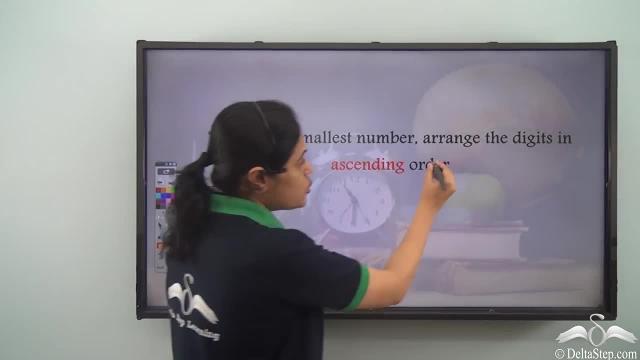 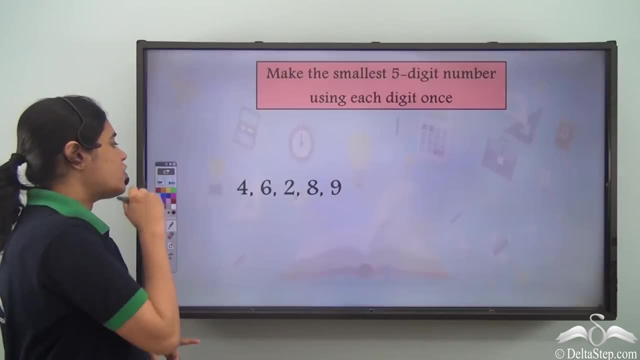 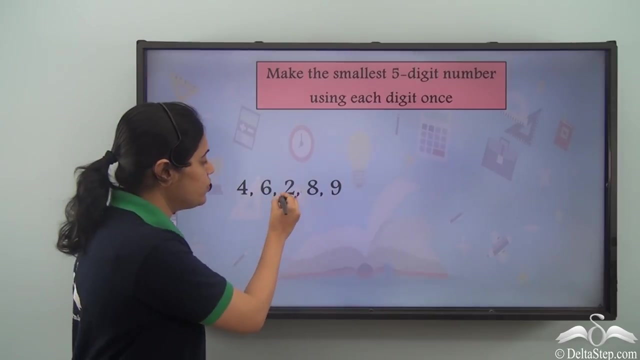 arrange the digits in descending order. So to make the smallest number, we need to arrange the digits in ascending order, That is, starting from the smallest, we need to move on to the largest digit. How can we do that? Which is the smallest digit here? 2.. So I start with. 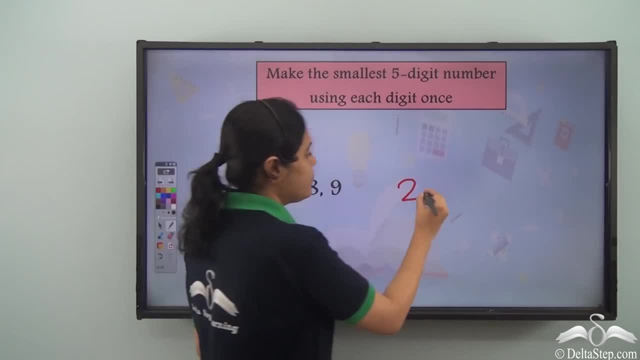 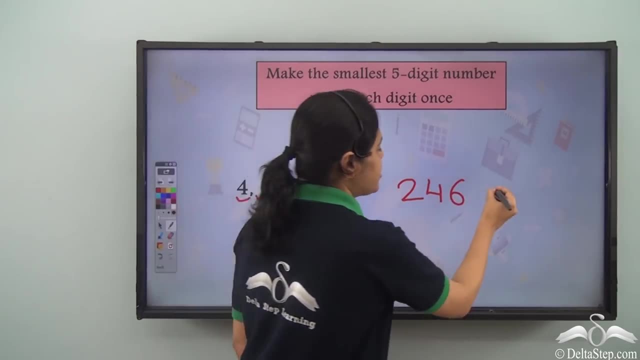 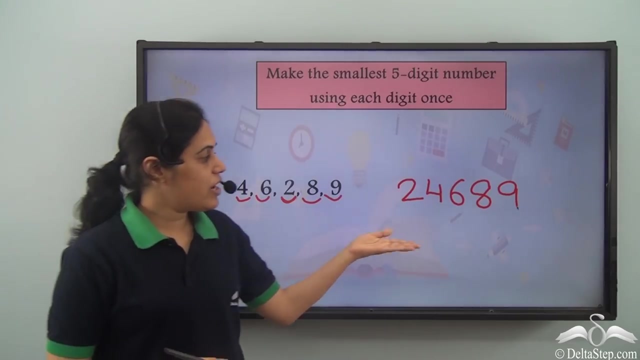 2.. The next digit is 4., So I write 4.. The next digit is 6., So I write 4.. The next digit is 7., So I write 6.. The next digit is 8., So I write 8.. And the next digit is 9., So we. 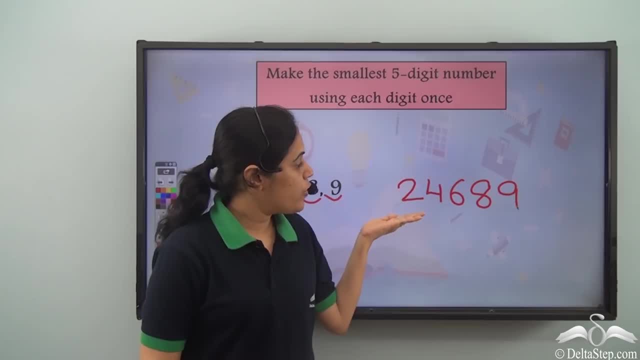 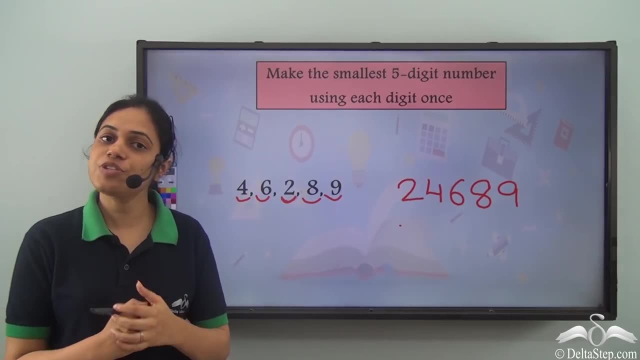 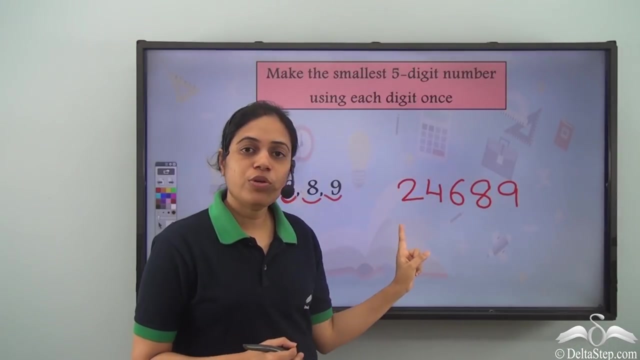 arrange the digits in ascending order: 24689.. This is the smallest 5 digit number that I can make using these digits. Now the logic is very similar to what we did for greatest number: We want to assign a lower value to the lowest digit number, So we want to assign. 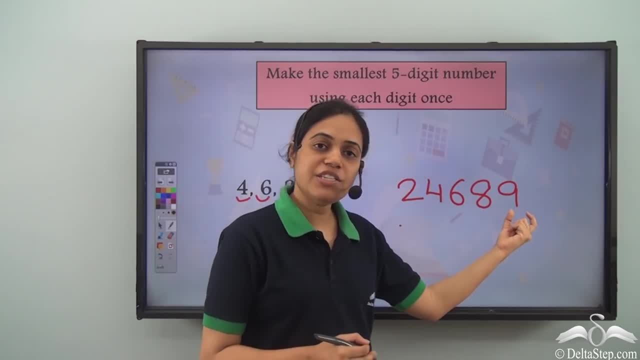 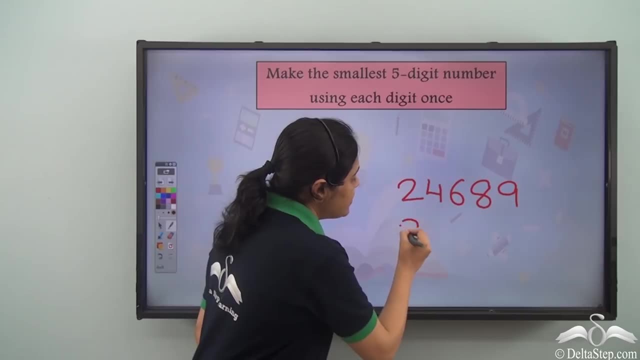 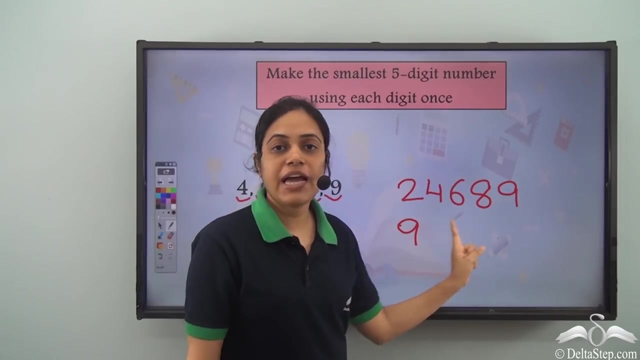 a lower value to the lowest digit number. So we want to assign a lower value to the higher digit because I want to make a smaller number as small as possible. So if I write this 9 here, I will get a greater number, because I know that for any two 5 digit numbers the 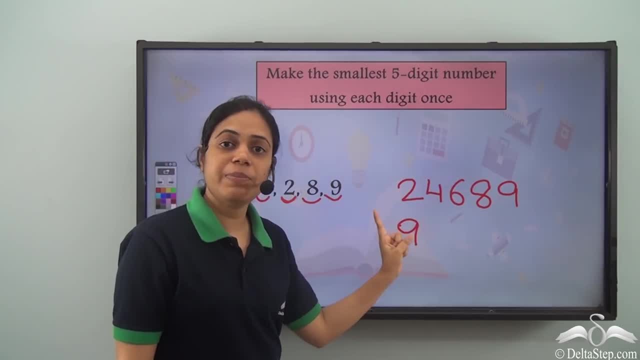 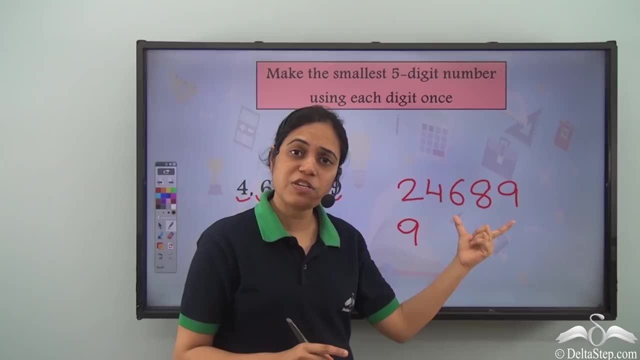 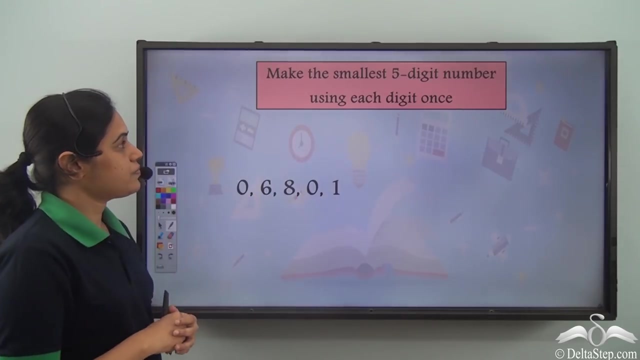 one having 9 in the 10,000th place will be greater than the one having 2 in the 10,000th place. But I want to make the smallest possible, So I arrange the digits in ascending order. Now, what about this one? I need to make the 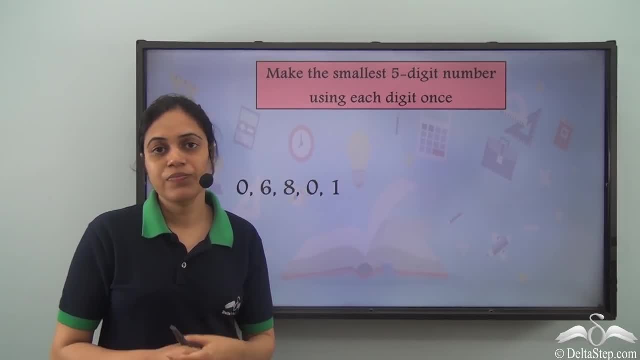 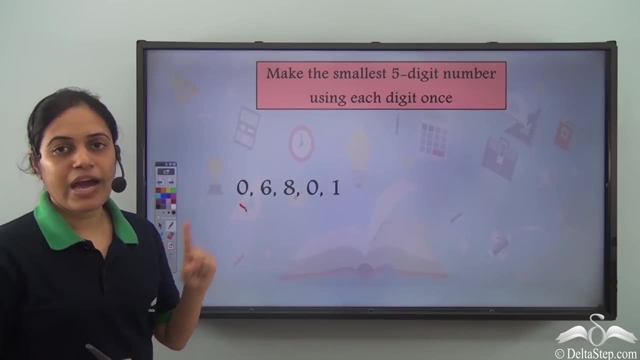 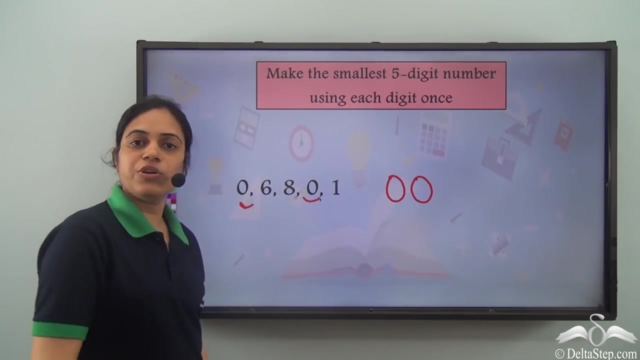 smallest 5 digit number using each digit just once. So let us arrange the digits in ascending order. The smallest digit is 0 and we have two 0s, So let us write 0s. So 1, 0, 2, 0. Then. 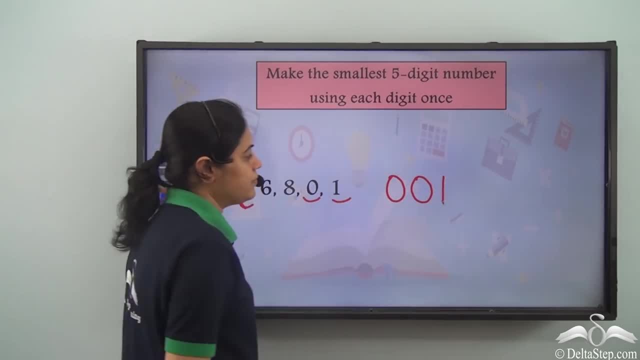 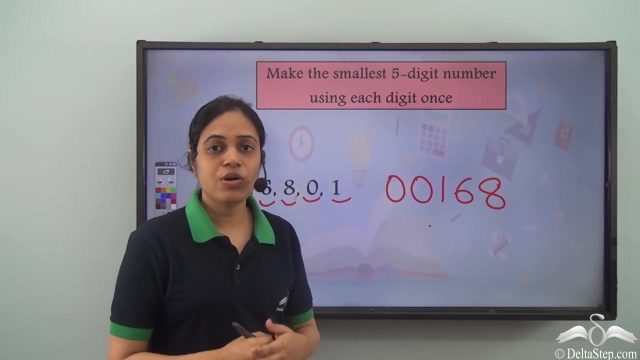 I have a 1., So I write a 1.. Then I have 6., So I write a 6. And then I have 8.. So these are the digits arranged in ascending order. But now look at this number. What is the number? 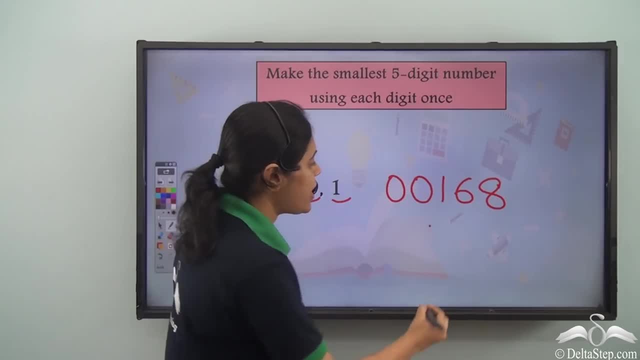 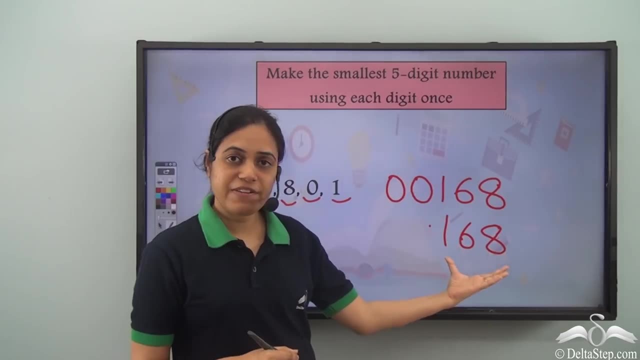 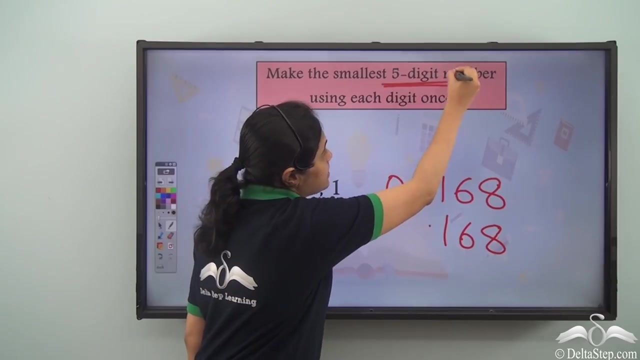 The number is 00168.. Or I can simply write this as 168.. Now, is this a 4?? Yes, it is a 4.. So I write a 4.. So I write a 4.. Is this a 5 digit number? No, This is a 3 digit number, Whereas what I want to make is: 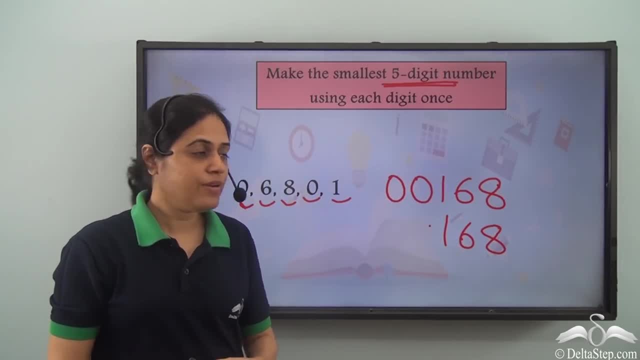 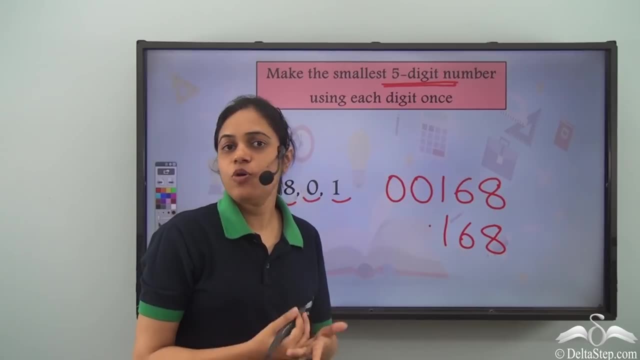 a 5 digit number. Why did this happen? Because we had 0s here And if I write 0 at the left, it holds no value, So we can ignore those 0s. So when you want to make the smallest number from the given digits and you are arranging- 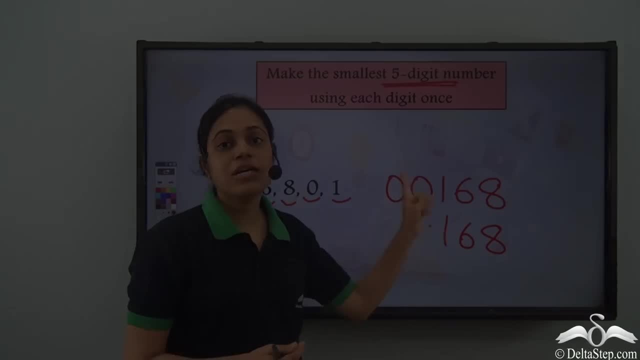 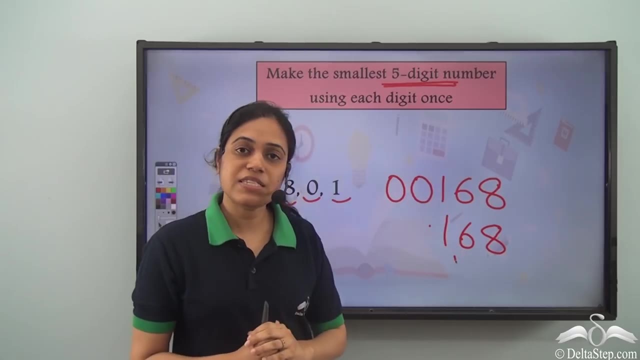 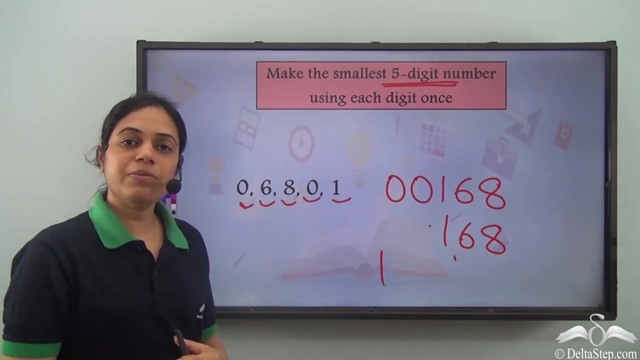 digits in ascending order. If there are 0s, the 0s will be written after the next largest digit after 0, which in this case is 1.. After 0, I have 1.. So the first digit of my number. 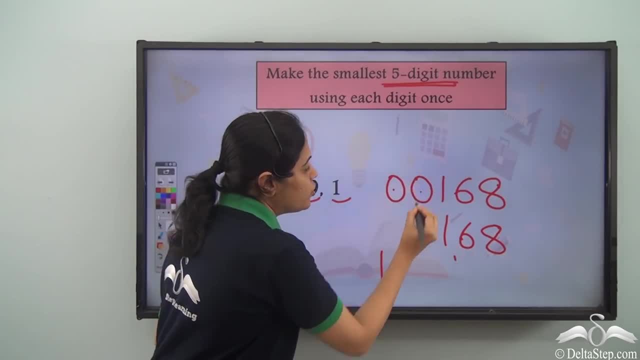 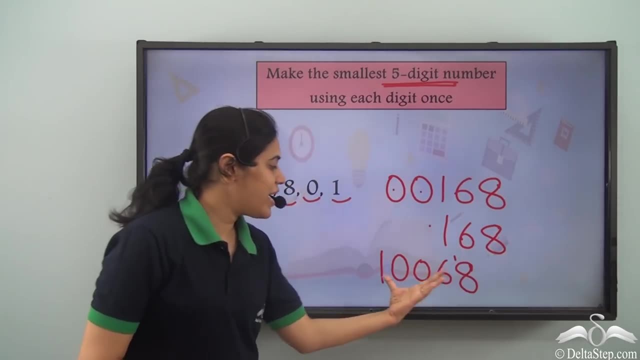 will be 1.. Then I write the two 0s, Then six and then eight. This is how I can make smallest 500, if get it typically TOOL digit number using these five digits. So instead of writing zeros to the left, I simply 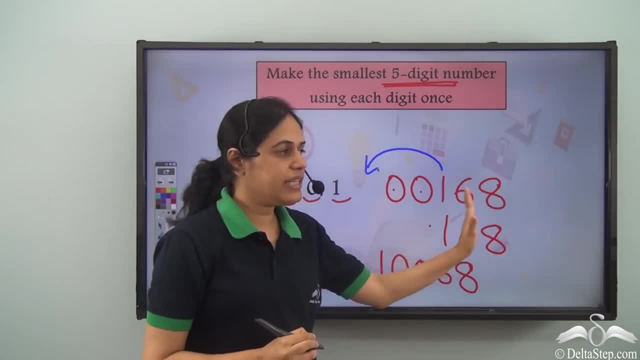 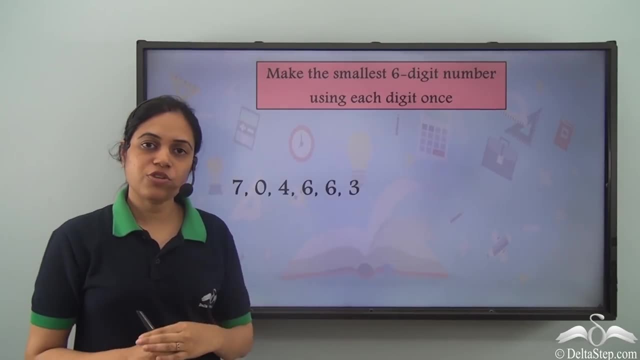 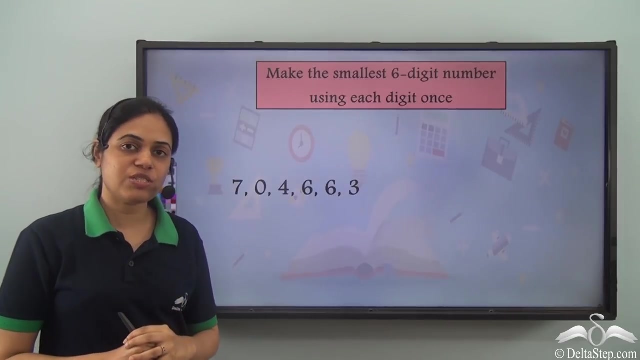 bring this one to the left, and all the other digits remain where they are. Now can you try this on your own? So we need to make the smallest six digit number using each digit just once. Now the smallest digit is zero, But now we know that we don't write zero in. 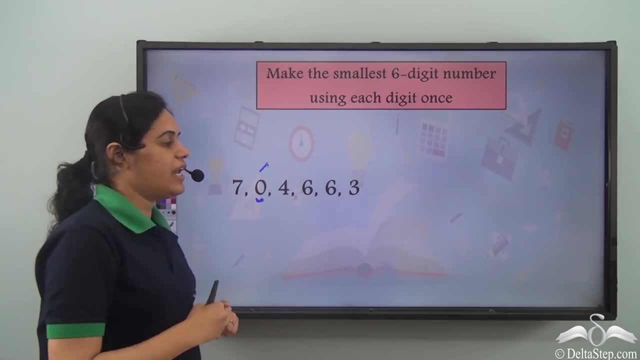 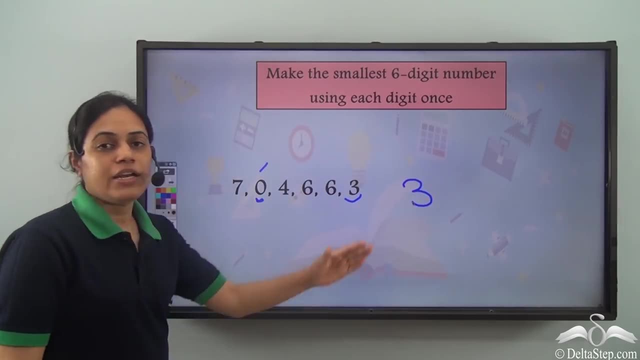 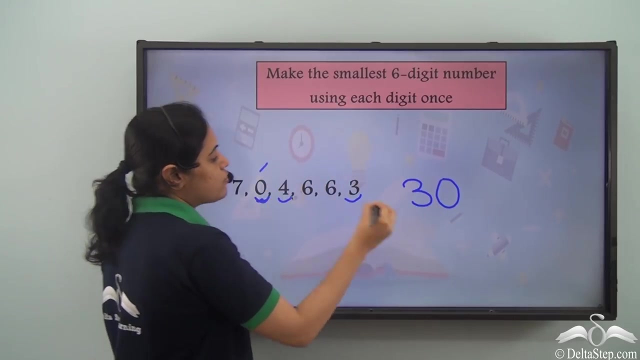 the beginning. So I leave this aside and move to the next digit, which is three here. So I write three first. Now I come back to zero and I write zero. The next digit is four, Next we have six. 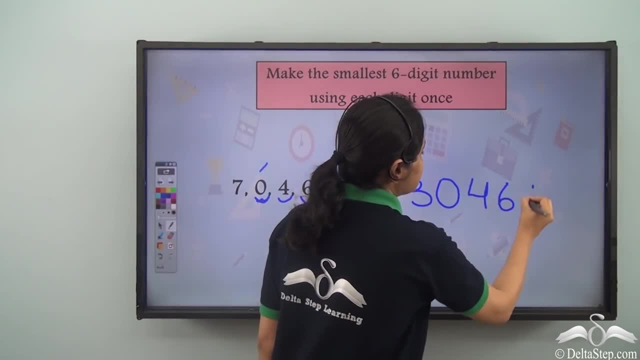 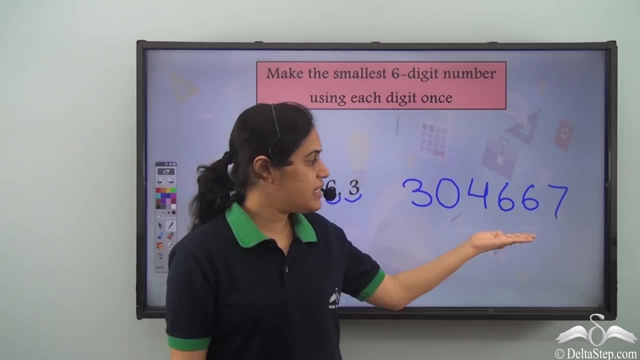 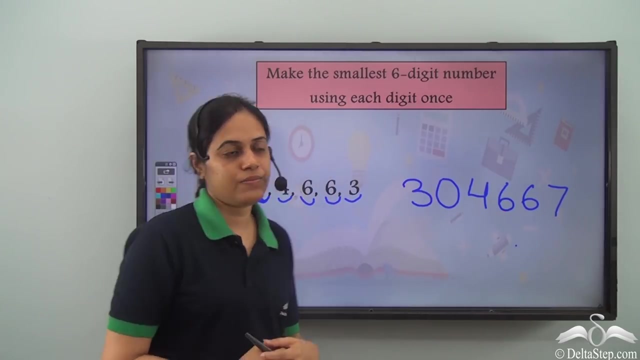 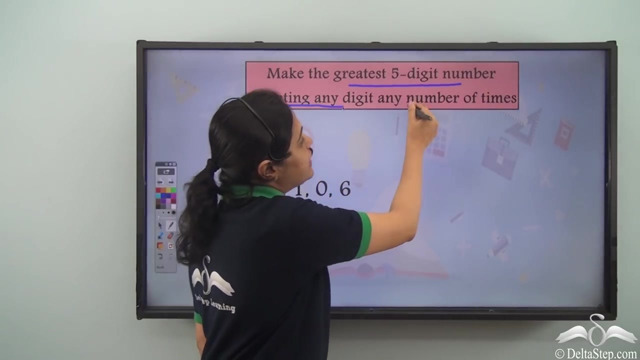 Six two times. So I write six two times and next we have seven. So this is how we can write the smallest six digit number from the given digits: 304667.. Now I need to make the greatest five digit number, repeating any digit any number of times. So till now we 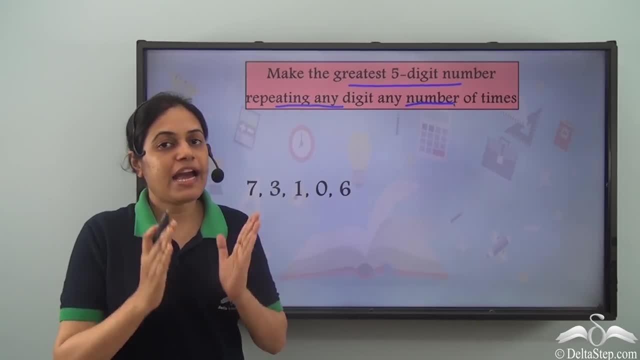 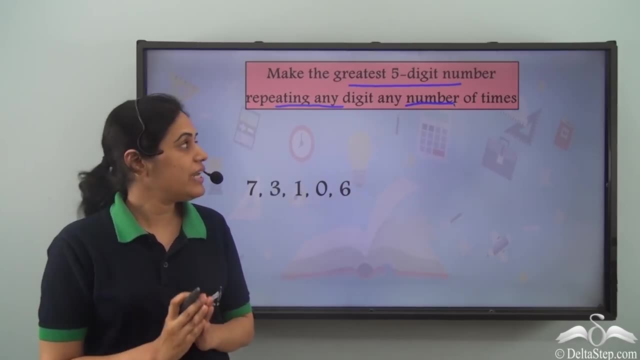 were not repeating any digits. Now I need to make the greatest five digit number, repeating any digit any number of times. We were always using every digit just once, But now I am allowed to repeat a digit. So how can I make the greatest five digit number using? 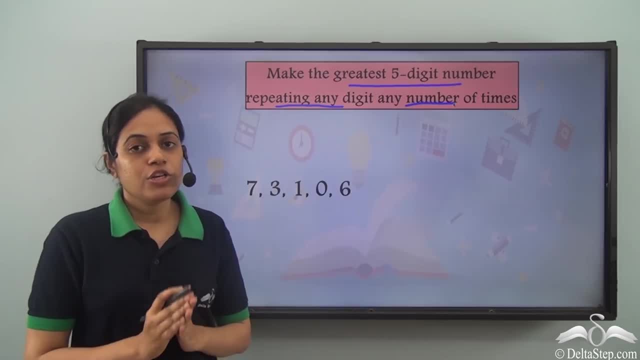 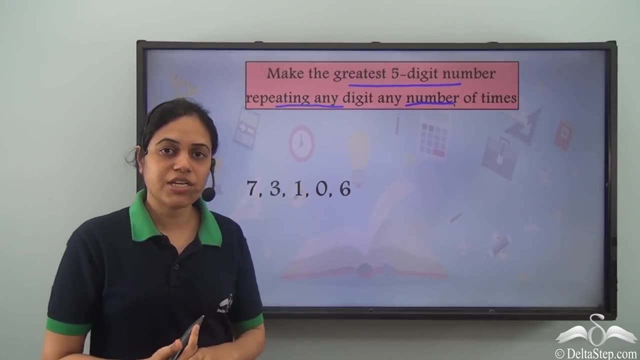 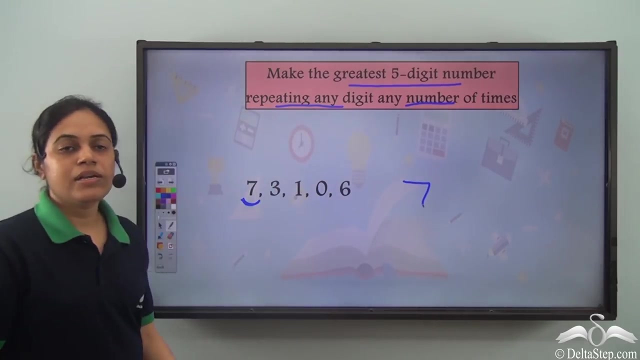 these digits with repetition. So I know that for making the greatest five digit number I need to start with the largest digit. The highest or the largest digit here is seven, So I write 7.. then I move on to the next digit. 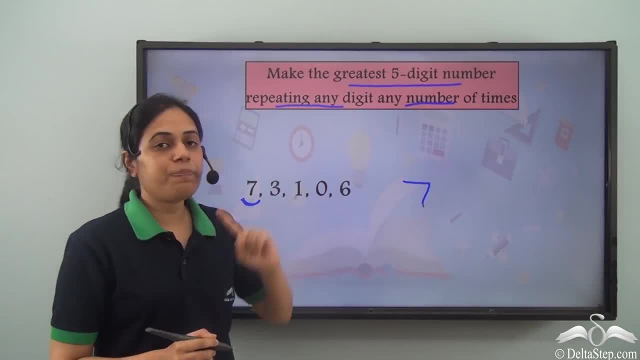 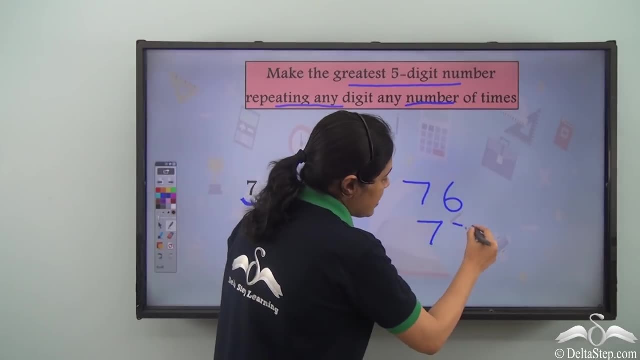 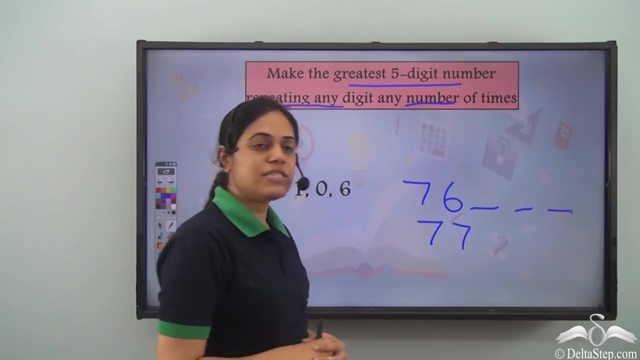 which is 6, but now I am allowed to repeat any digit. so if I write 6 here versus if I write 7 here, then this number will be greater. this will be a five digit number. this will be a five digit number. now I know that if the digits in ten thousands, 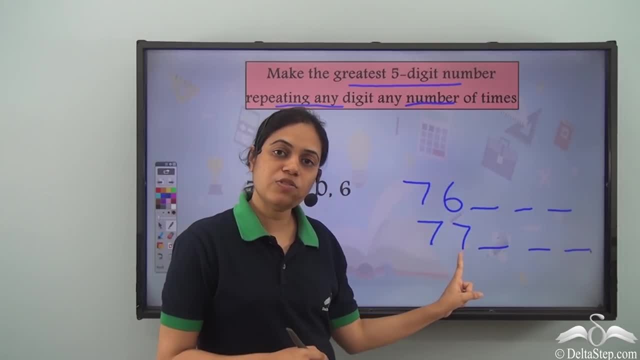 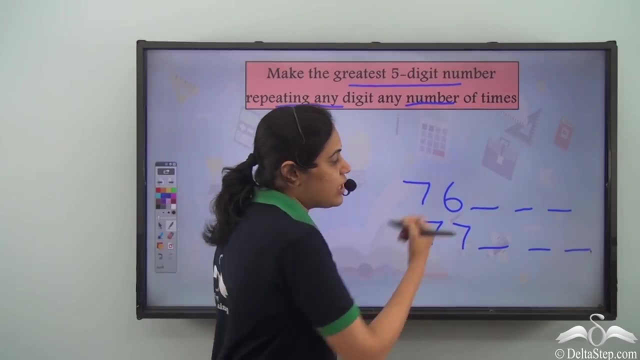 place are equal. I need to compare the digits in the thousands place. in the thousands place, if I have 7, this number will be greater than this number where I have 6 in the thousands place. so I will write a 7 here now once again. what will come here I will write. 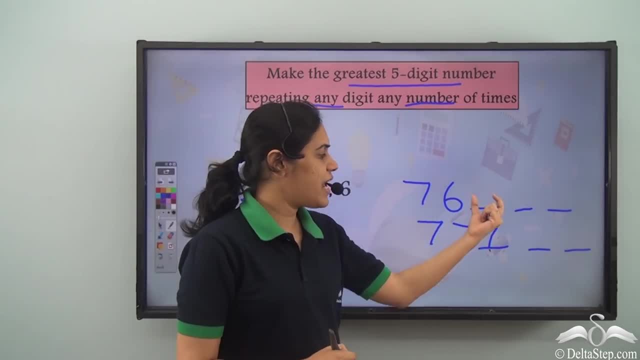 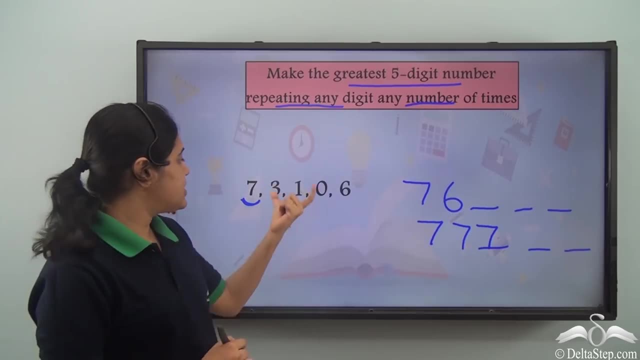 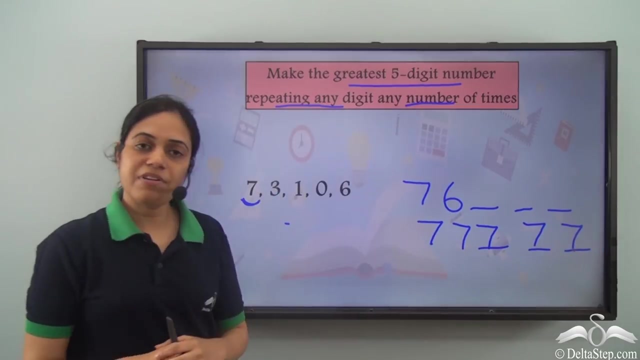 7 once again, because if I write any other digit then that number will be smaller than if I write 7, because 7 is the highest digit that I can get. similarly, I'll have 7 here and 7 here, so the greatest five digit number. 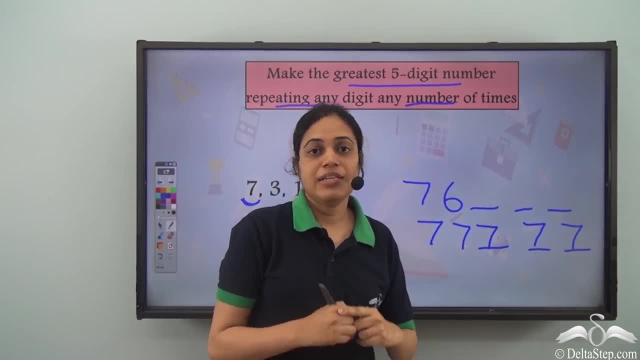 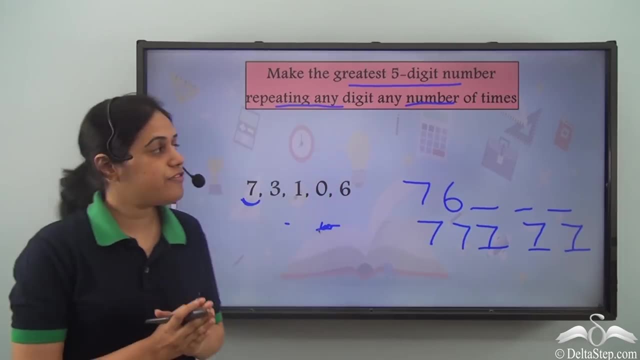 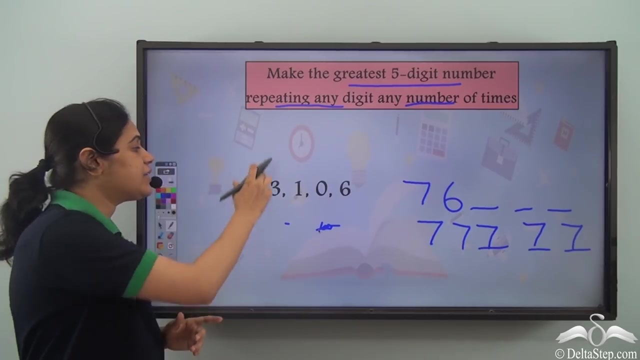 will be 77777, that is, 7 written 5 times 77777. so if we want to make the greatest five digit number, the greatest five digit number will be 77777. from the given digits, I need to repeat the highest digit 5 times. 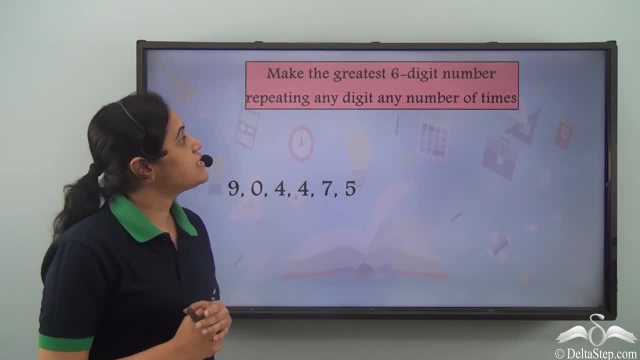 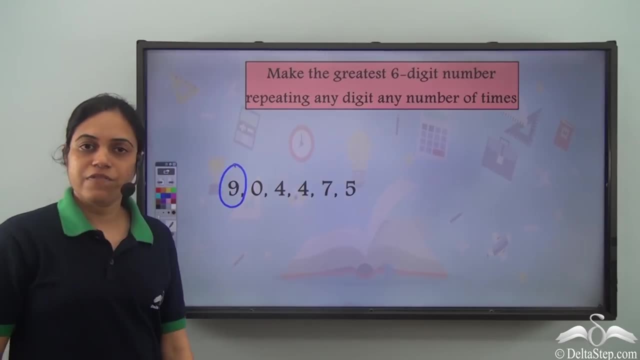 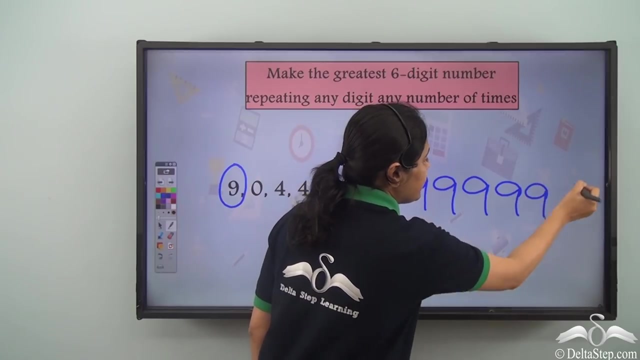 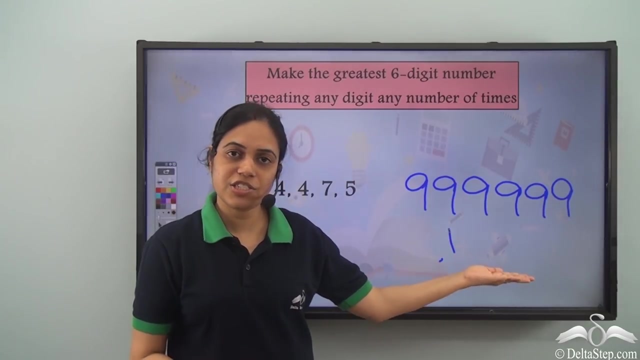 what about this? we need to make the greatest six digit number, repeating any digit any number of times. so once again, find the highest digit, which is 9, and write it 6 times 999999, 9. I already know that this, in any case, is the greatest six digit number there cannot be. 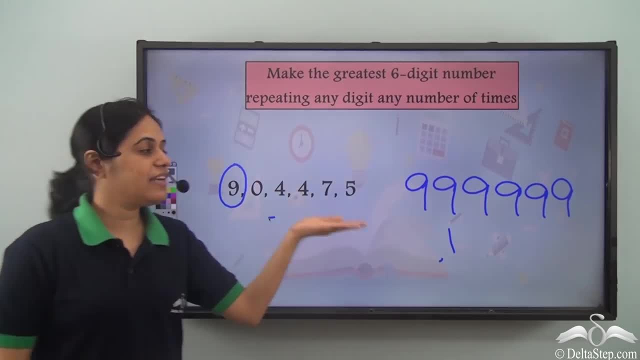 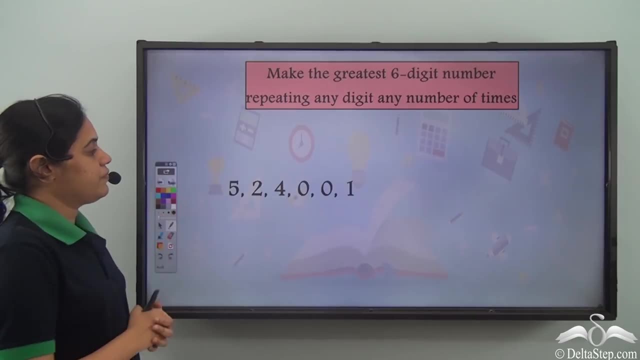 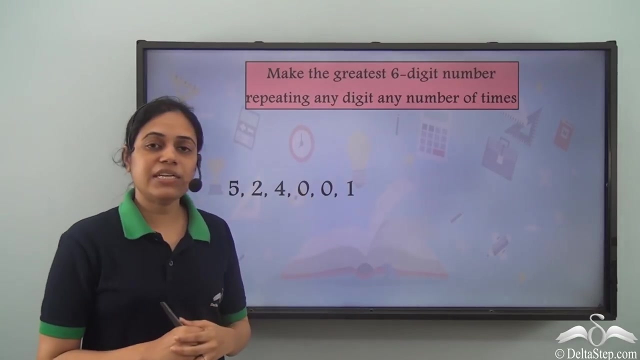 any other six digit number which is greater than this and given the digits as well, this is the greatest six digit number which we can make. so now can you try this on your own. once again, I need to make the greatest six digit number by repeating any digit any number of times. 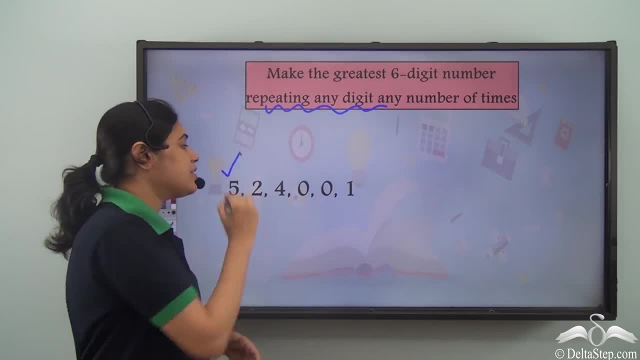 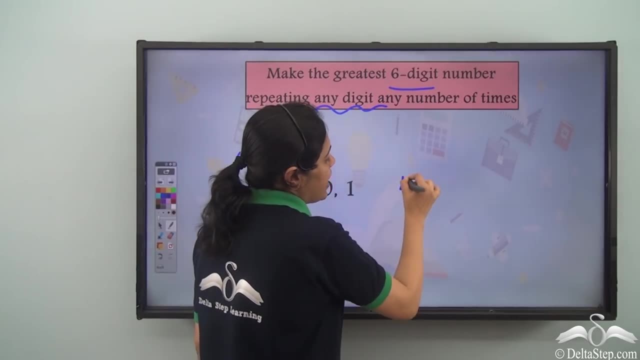 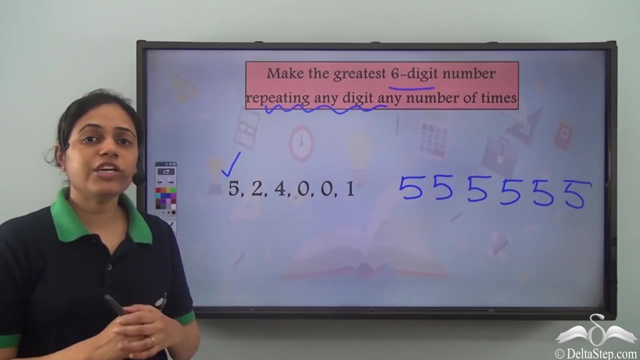 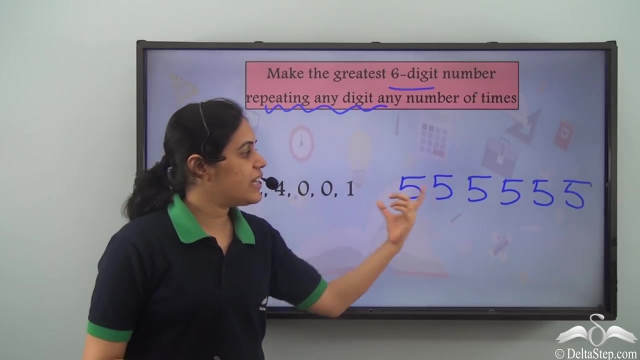 so the only thing that I need to do is find the greatest digit, which is 5. here, and because I need to make a six digit number, I write 5 6 times. so you can try it on your own. you can use any other number, you can take any other combination and you will see that this 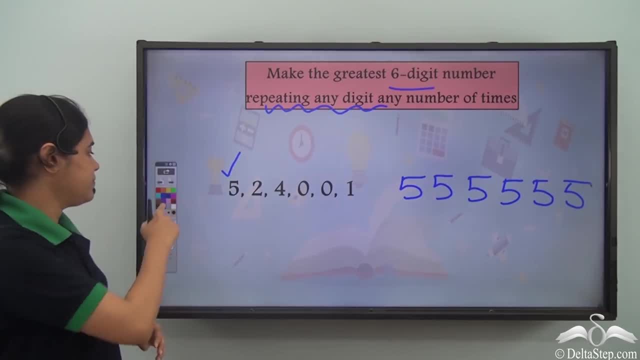 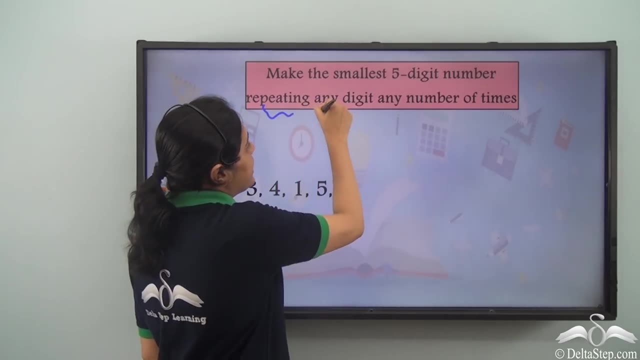 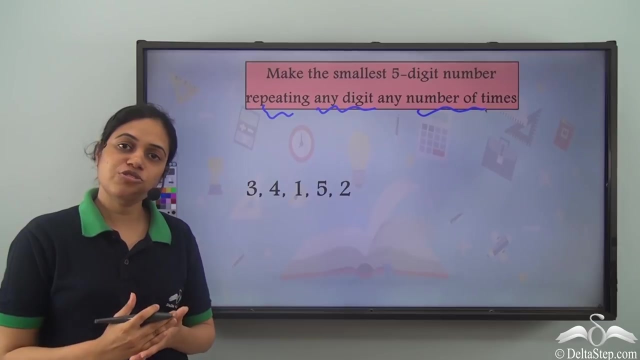 is the greatest number that you can get. now, how do I make the smallest five digit number, repeating any digit any number of times? so when I was making the greatest number, I was using the largest digit. now I need to make the smallest number, so I will choose the smallest digit. 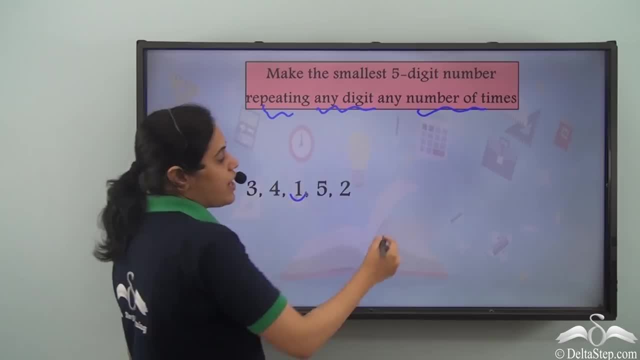 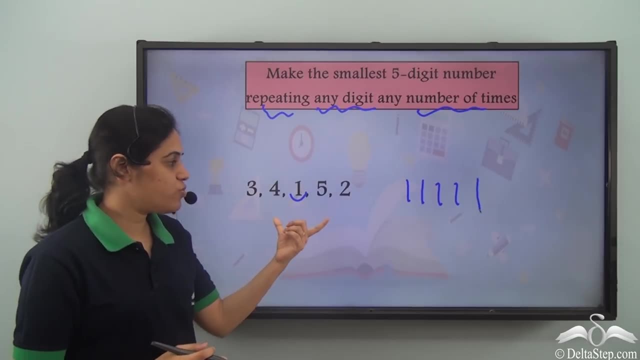 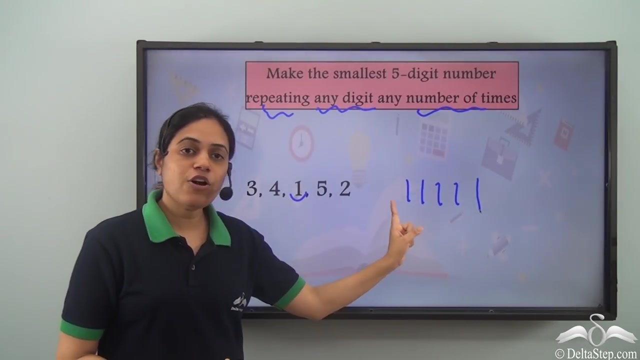 the smallest digit here is 1, so I write 1 five times. this is the smallest five digit number which we can make using these five digits. if I use any other digit in place of 1 in any of the places, then that number will be greater than this number. 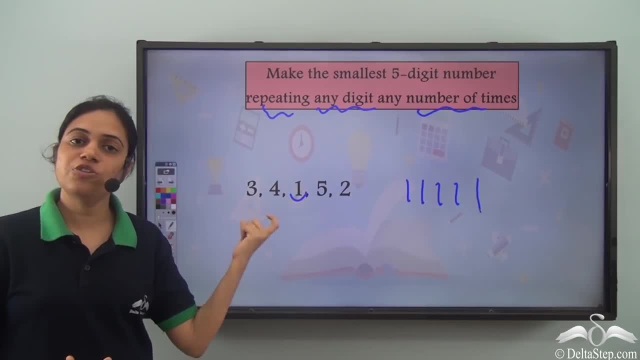 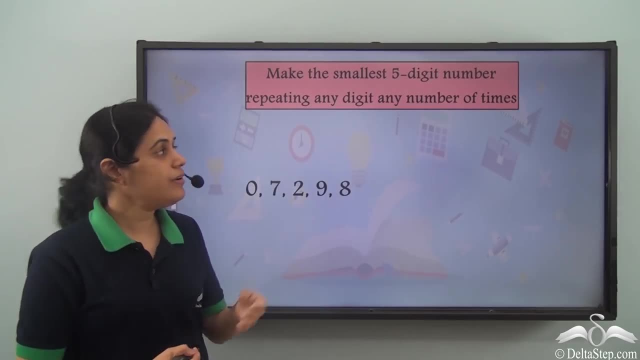 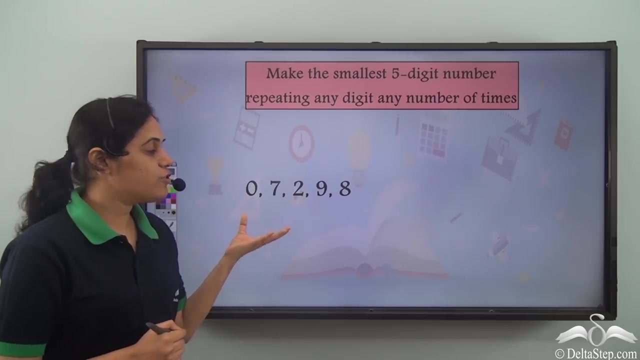 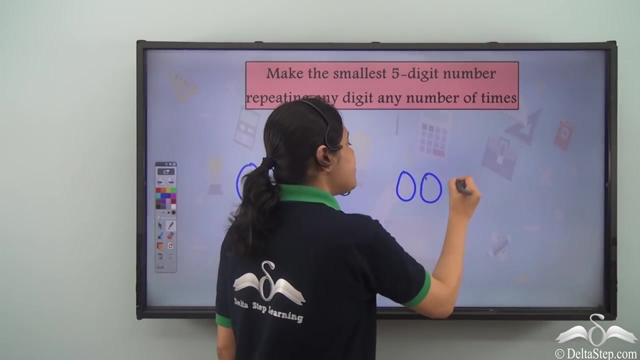 so this is the smallest number which we can make using these digits. now, what is the smallest five digit number that we can make using these digits with repetition? so once again, I need to find how do I find the smallest digit. The smallest digit is zero, so do I write 0, 5 times? 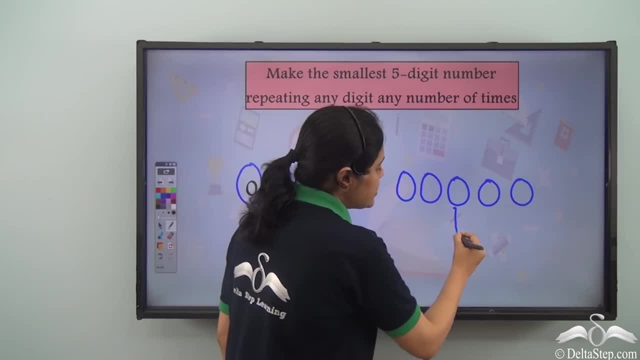 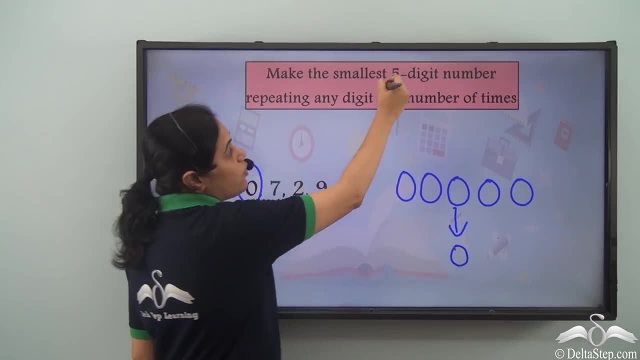 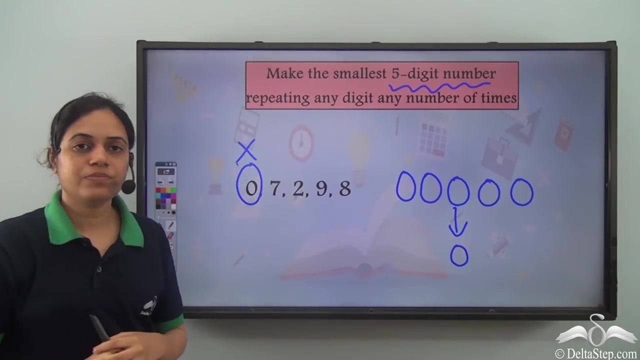 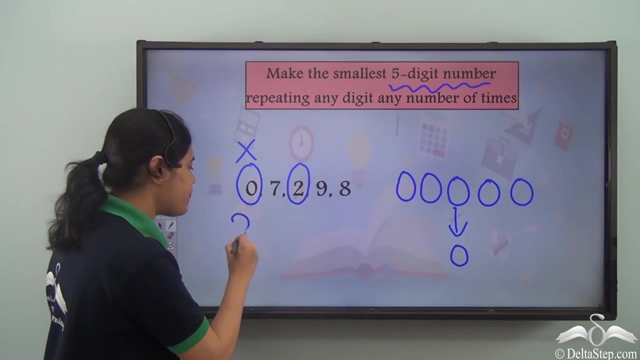 and say that this is the smallest five digit number. no, because this, this is simply equal to zero and this is not a five-digit number, whereas what I want is a five digit number and I choose 2.. So what do we do? We write 2, 5 times, But is this the smallest 5 digit? 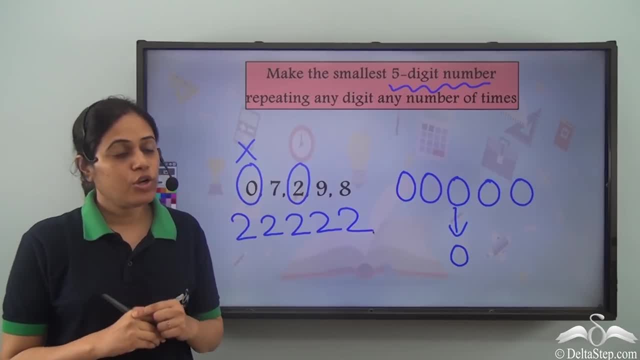 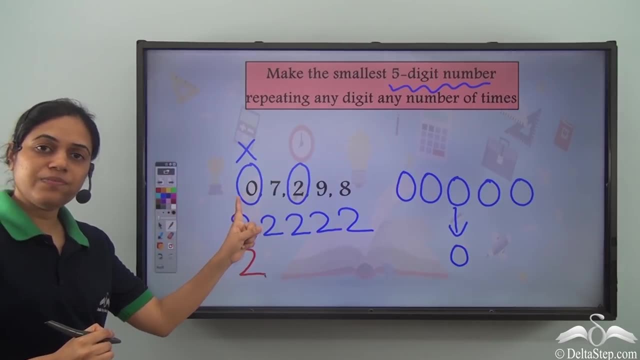 number that we can make using these 5 digits? No, because I write 2 first, then I have 0s here. 0 is less than 2.. So these 4 digits can be written as 0s. I can't write 0 in the. 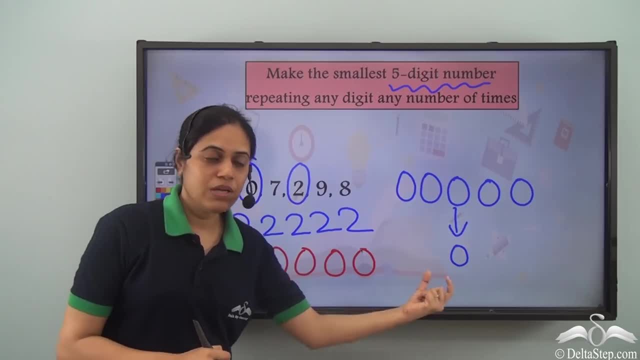 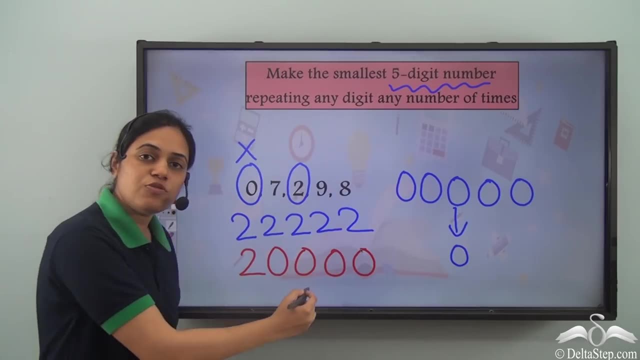 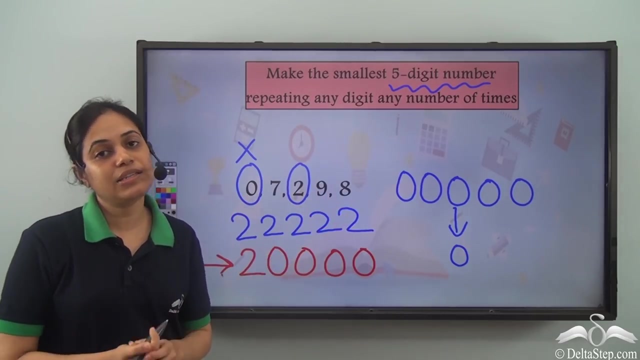 first place, because then the number will become 0. But I can write 0s to the right of 2. So the number will become 20000.. And this is the smallest 5 digit number that I can make using these 5 digits, So 2.. 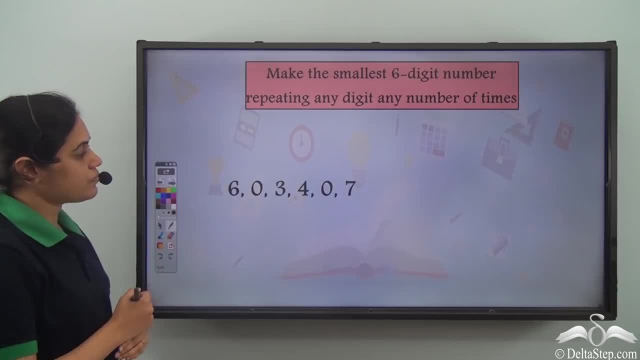 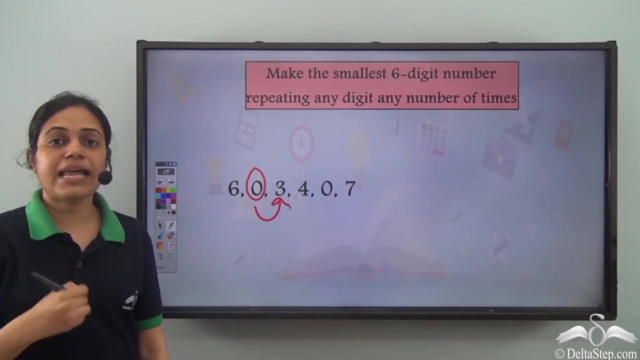 Followed by 4, 0s. And now can you make the smallest 6 digit number using these digits? So I have 603407.. So the smallest digit is 0 here. But I will not start with 0, because I cannot start a number with 0. So I go to the next digit, the next largest digit after. 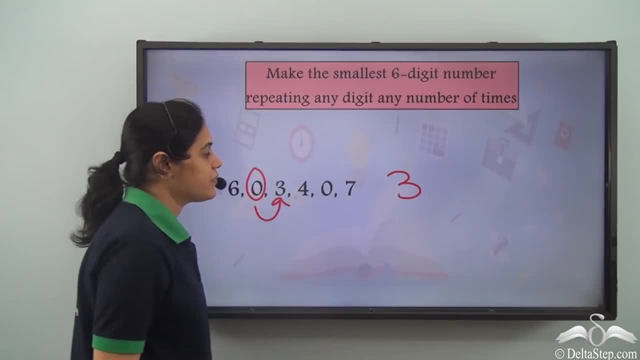 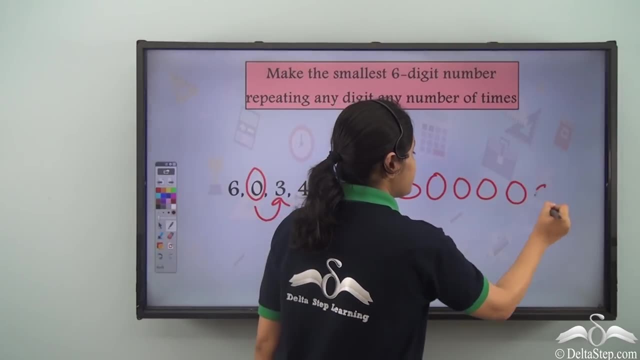 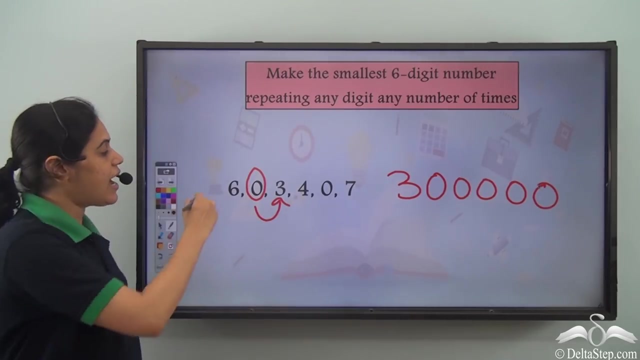 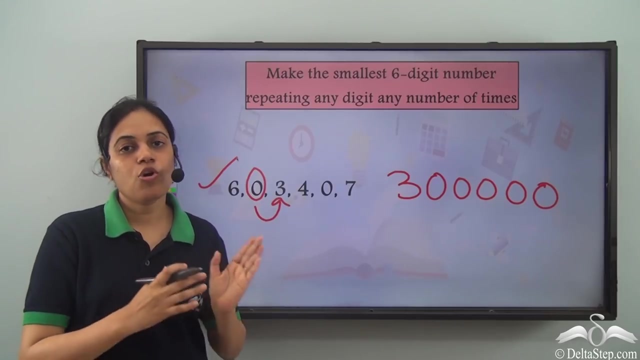 0, which is 3.. So I write 3 here And then I come back to 0 and I write 5: 0s. So 3 lakh. 3 lakh is the smallest 6 digit number that I can make using these 6 digits. So this is how you can make the greatest, or? 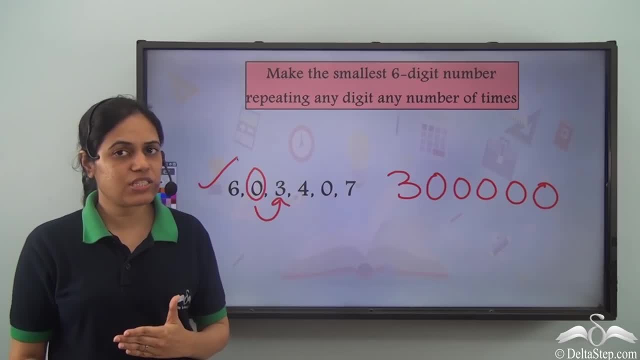 the smallest numbers: greatest 5 digit or 6 digit. smallest 5 digit or 6 digit numbers using the greatest number. Now, now we come back here: 0.. Now you see, halfway through, the problem is here also, I have done both numbers, But it is all wrong. Well, I know that I 0001;. 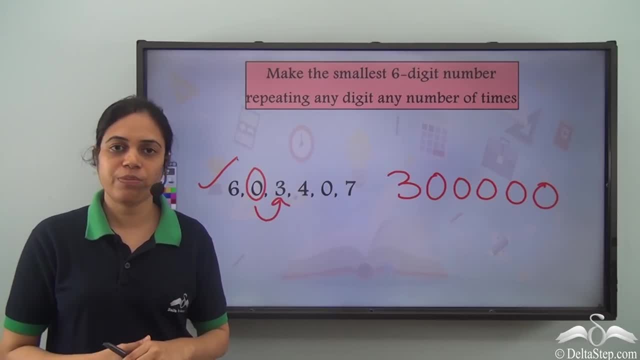 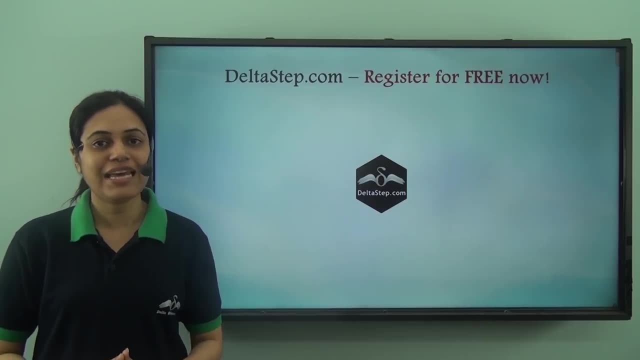 given digits with repetition or without repetition. If you like this video, then subscribe to our channel. You can also register for free at deltastepcom to get all the learning resources as per CBSE, ICSE, IB, Cambridge or any other. 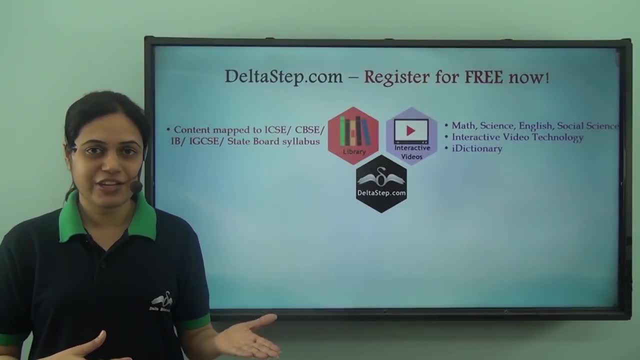 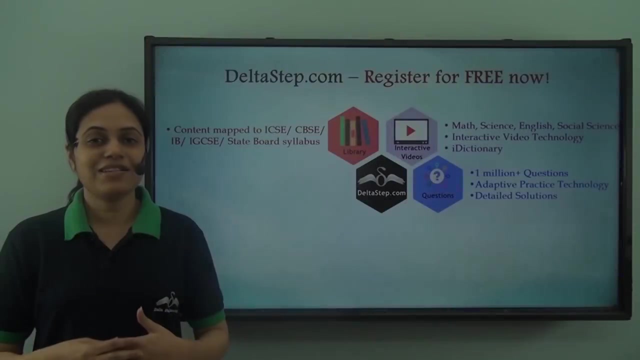 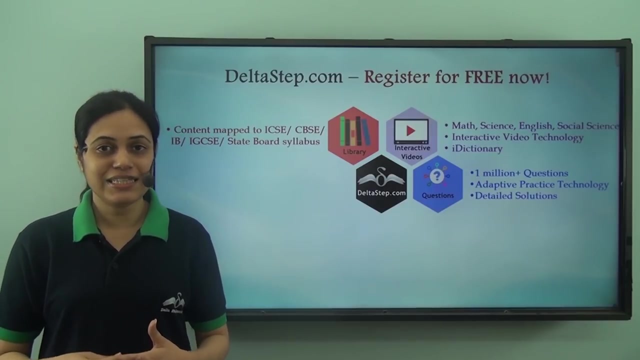 curriculum: Over 5000 amazing lectures on Maths, Science, English and Social Science. Our unique interactive video technology keeps you engaged and our iDictionary feature allows you to quickly revise any concept. Master each topic at your own pace with our adaptive practice technology and 1 million plus questions. Get instant answers and detailed solutions. 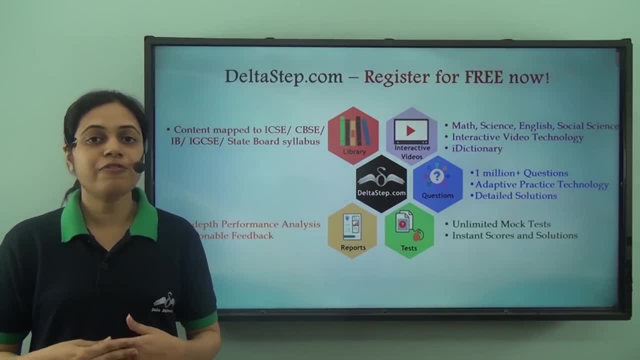 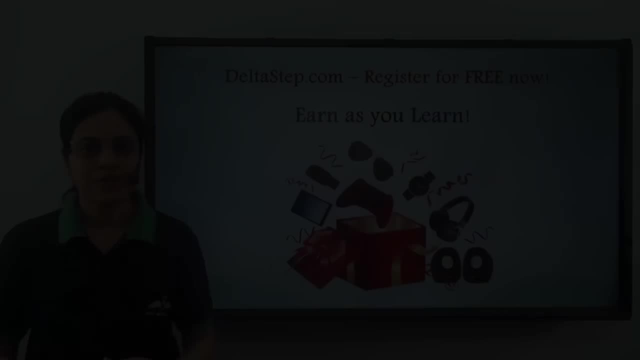 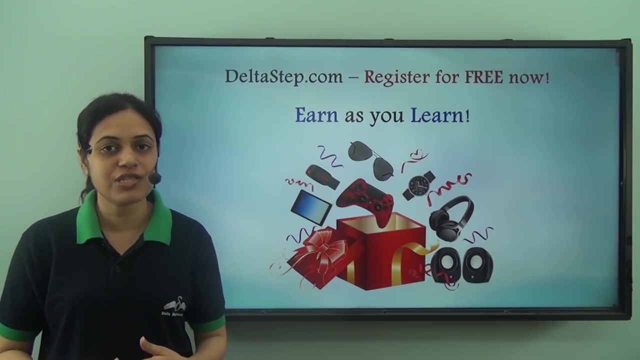 Be exam ready by taking unlimited mock tests, performance analysis along with actionable feedback, Personal tutors to resolve the slightest of your doubts. And that's not all. You can also win exciting prizes like PlayStations, iPads, watches and many more, along with certificates through our Earn as you Learn program. So at deltastepcom.